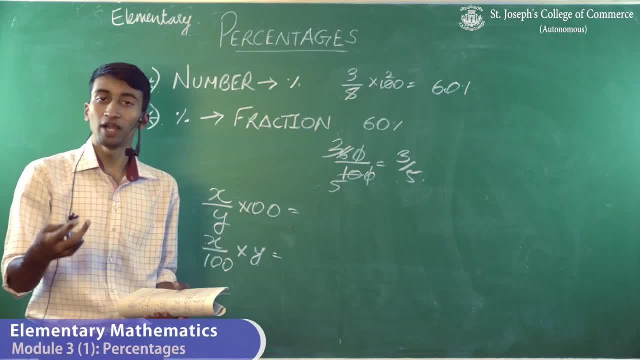 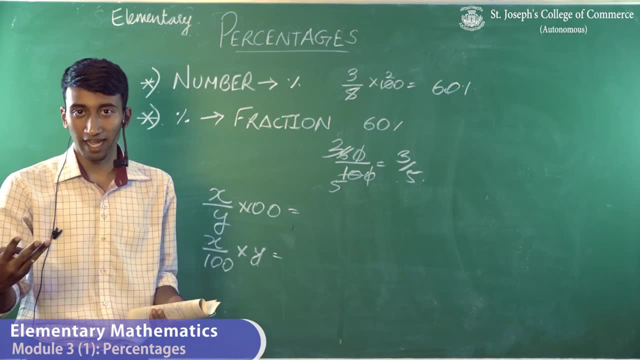 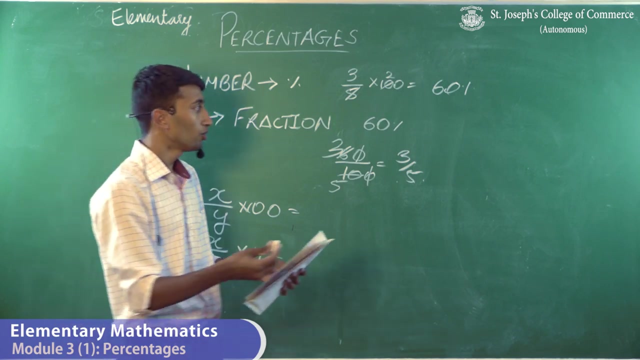 in a question they ask you. they tell you that you have 2 rupees and now you have 5 rupees, So there's an increase of 3 rupees as of now. So they ask you. so if the question asks you the increase percentage, all you need to do is find the increase of what you. 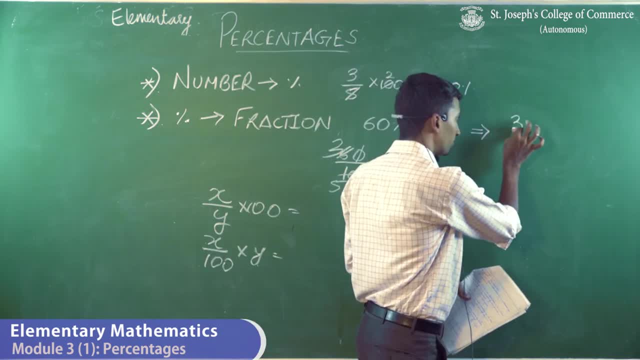 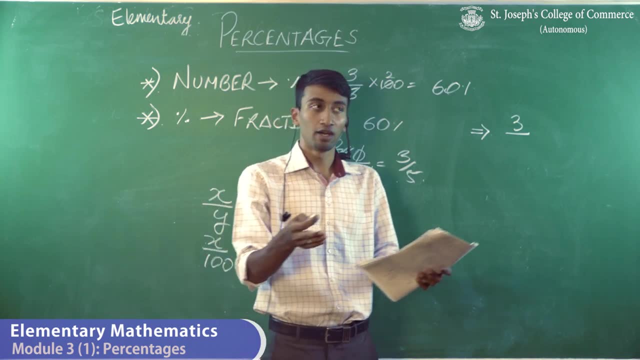 had. So what you have now that is 3 rupees, from 2 rupees to 5 rupees. So that's 3 rupees divided by 2 rupees. That is your previous holdings, the amount that you held before it increased. 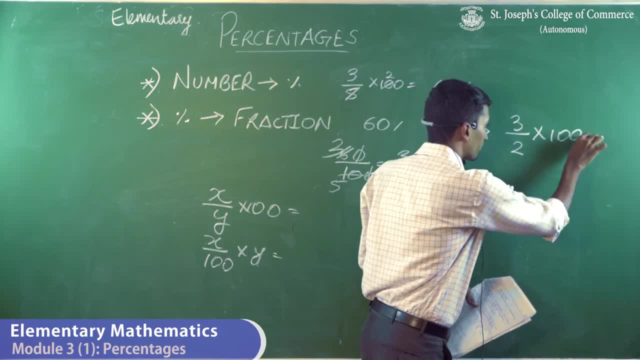 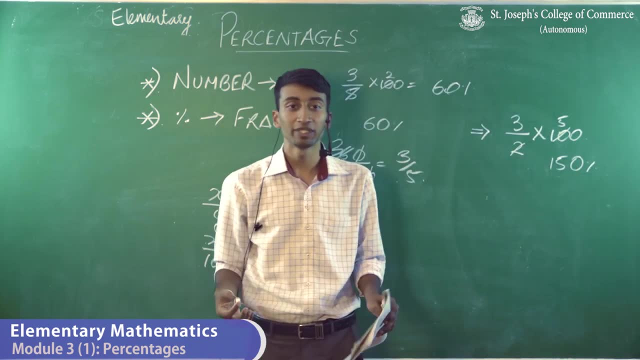 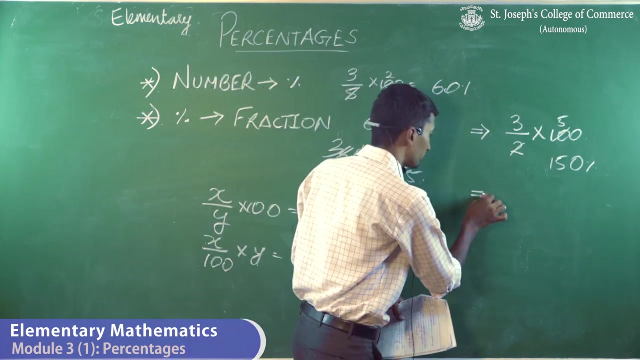 That is 2 into 100. And you get your answer. That would be 150%. So you have a 150% increase in what you're holding right now. The same way: decrease percentage. All you need to know is say, for example, you have 5 rupees and now you have only 3. 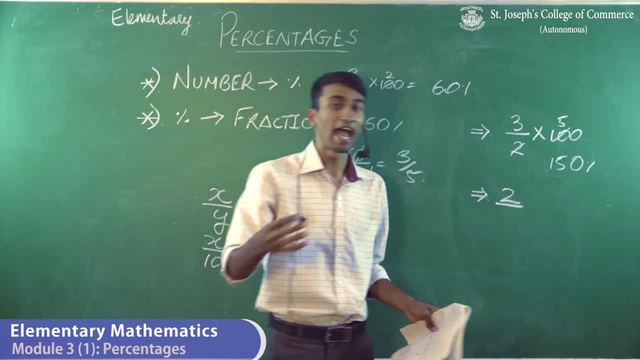 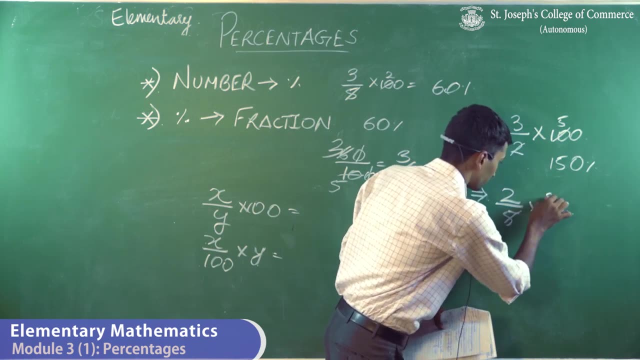 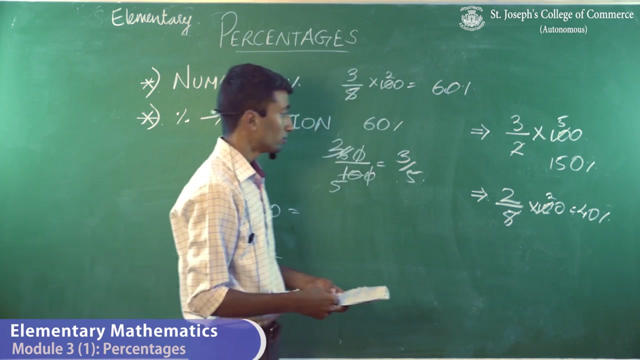 rupees. So your decrease is 2 rupees, and you had 5 rupees. So that's 2 by 5 into 100. So your holdings decrease by 40%. Now I'll give you an easy formula of how to do it That. 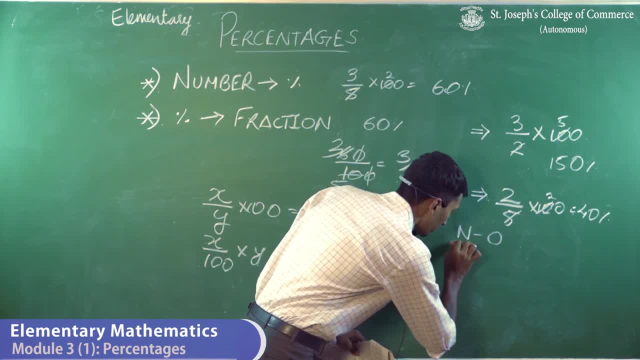 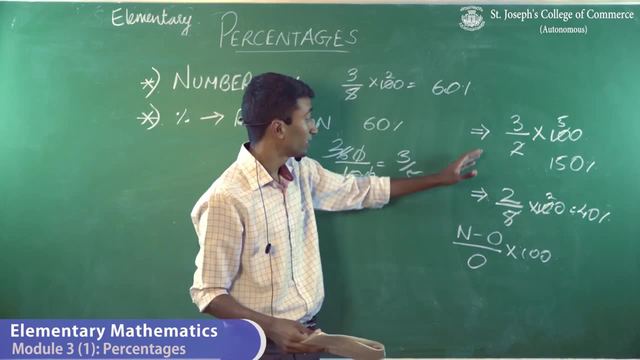 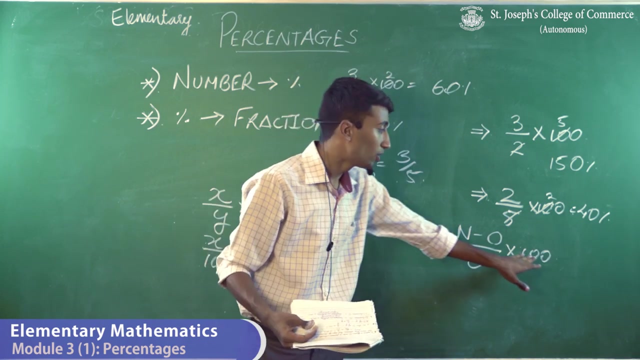 is new minus old by old into 100. So new earnings. So basically the new holdings that you have minus your old earnings, divided by your old earnings into 100. Normally when it's increased percentage and decreased percentage. this is what you remember. 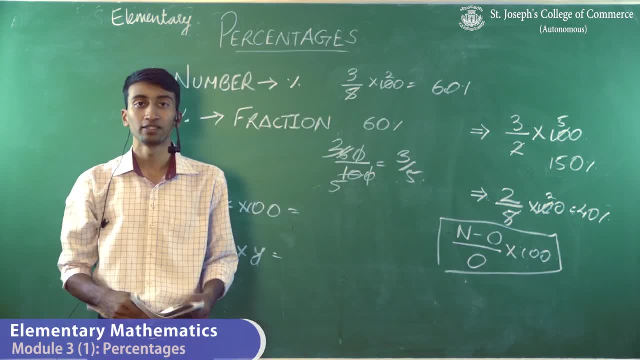 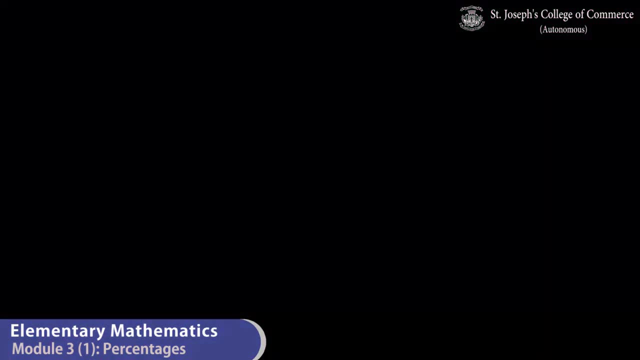 New holdings minus old holdings divided by old holdings will give into 100.. It will give you your percentage. This is about 3.3 per cent. So that's 3.3 per cent. So this is your, your increase or decrease percentage. so we now move on to the sums under percentages. 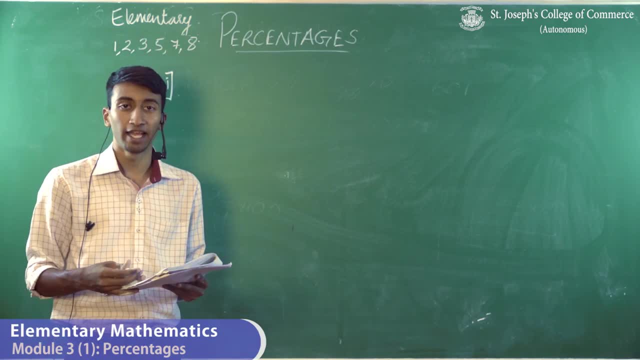 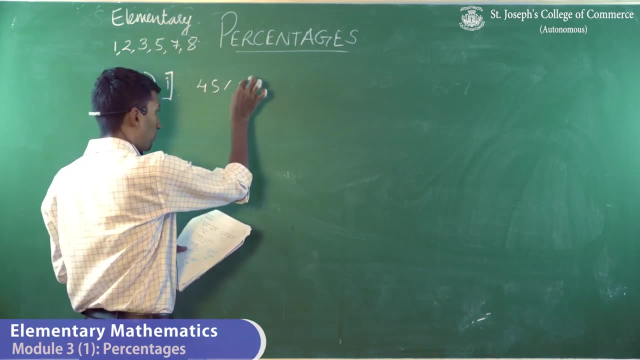 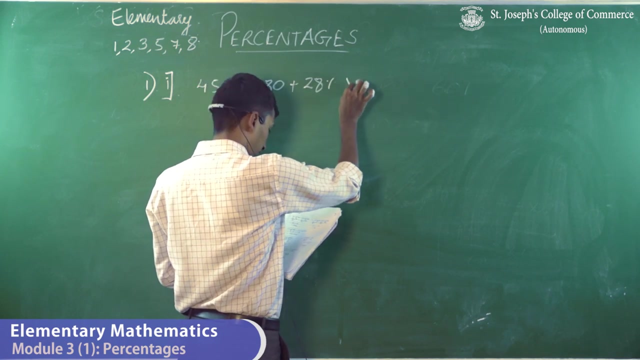 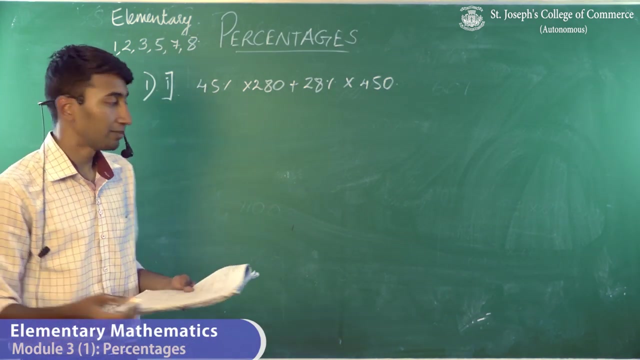 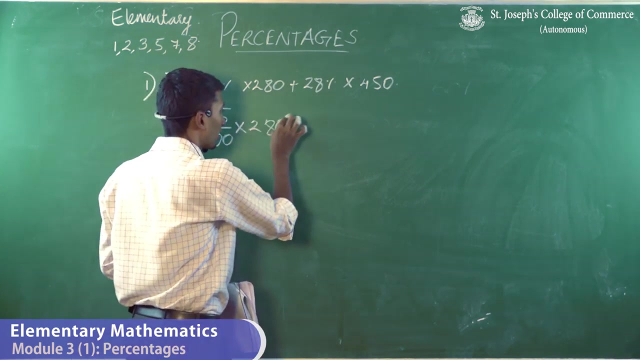 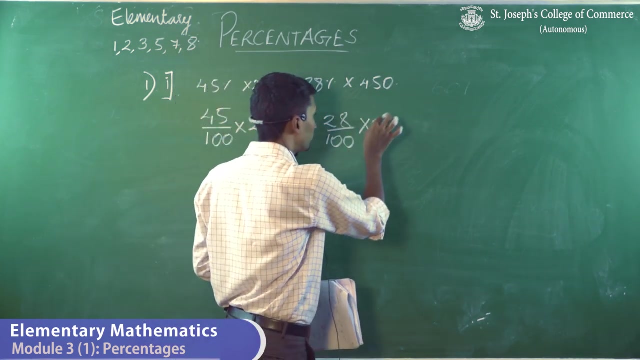 where we are going to solve the first, second, third, fifth, seventh and eighth sums. so the first sum under the first sum, the first part, that is 45 percent of uh of 280 plus 28 percent of 450. so now 45 percent of 280 means 45 by 100 into 280, and 28 percent of 450 is 28 by 100 into 450. 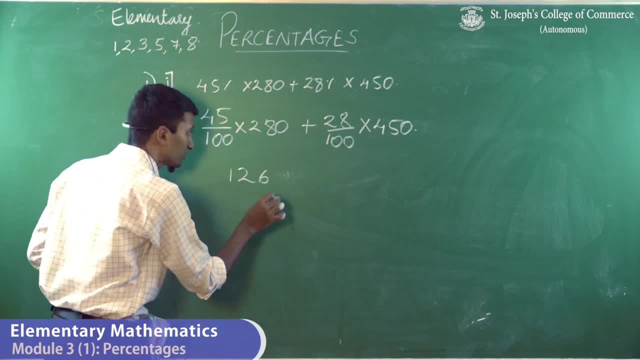 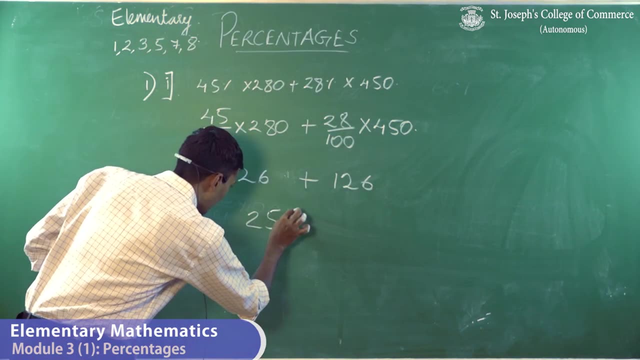 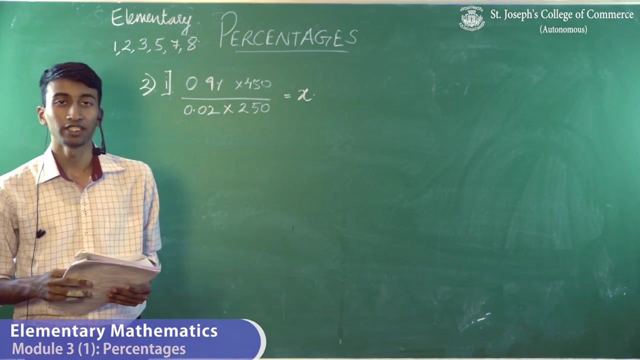 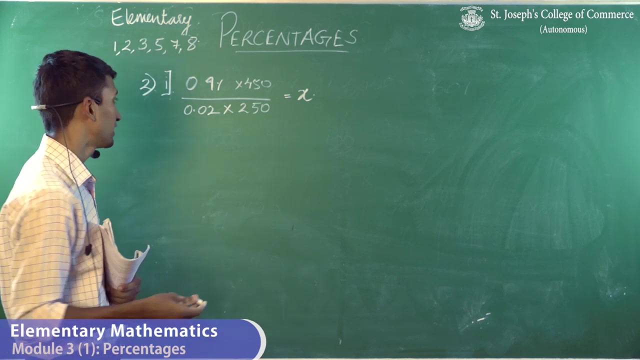 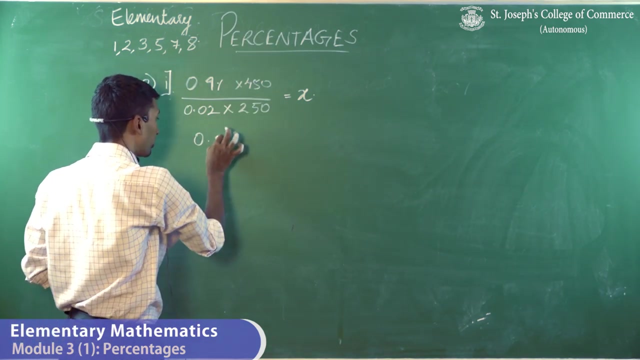 if you solve it, you will get 126 plus 126, which will be 252, as your answer. so, moving on into the second sum part one, uh, wherein the question says: 0.9 percent of 450 divided by 0.02 percent of 250, uh is x. so what we do over here is 0.9 by 100 into 450. 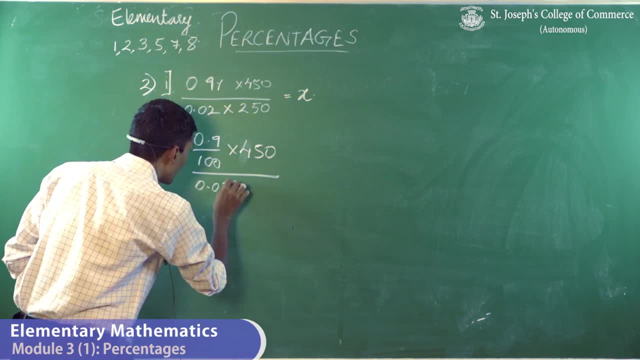 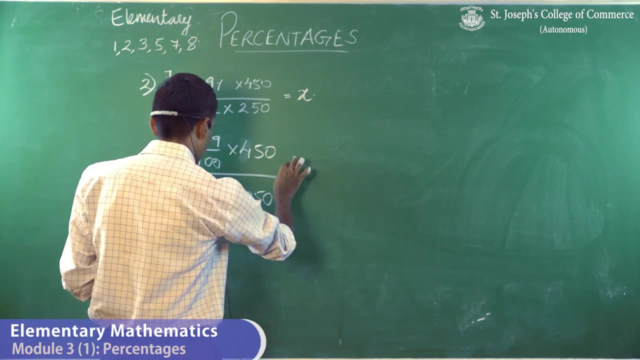 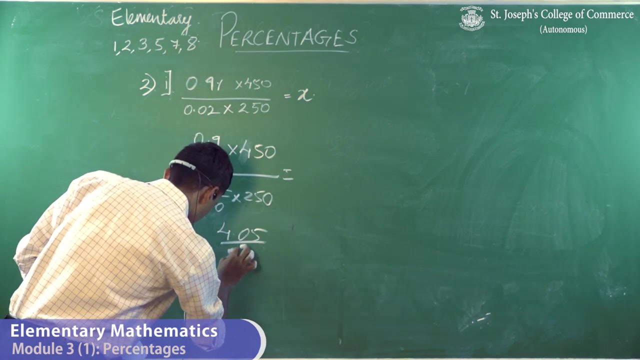 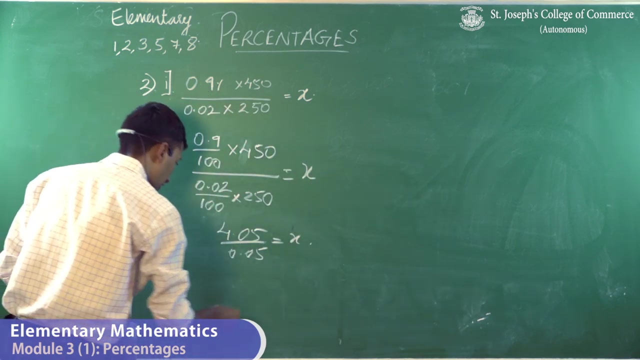 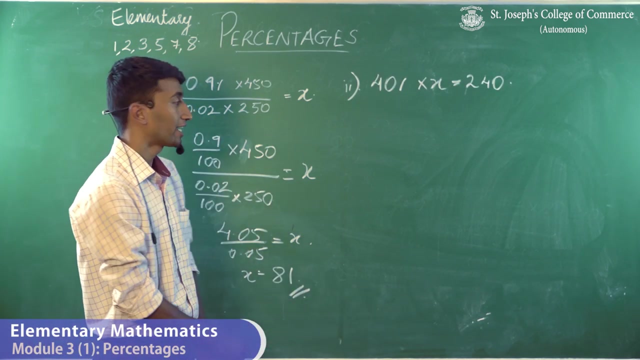 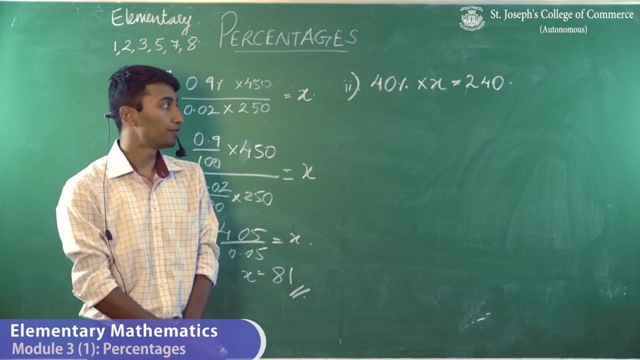 by 0.02, by 100 x 250.. so we get um say 4, 4.05 and 0.05 is equal to x. so then if we mu, if we simplify it again, we get 81.. as you are answer, Moving on to the second part of the question, the question says 40% of X is 240. 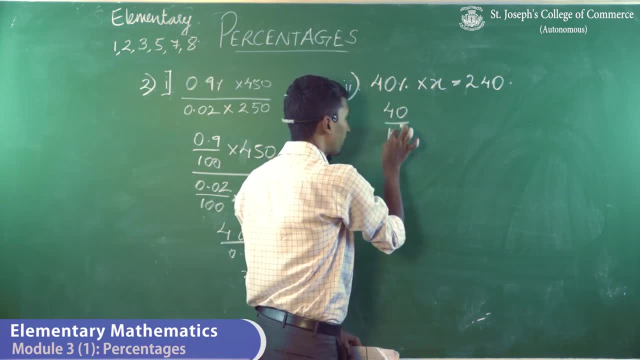 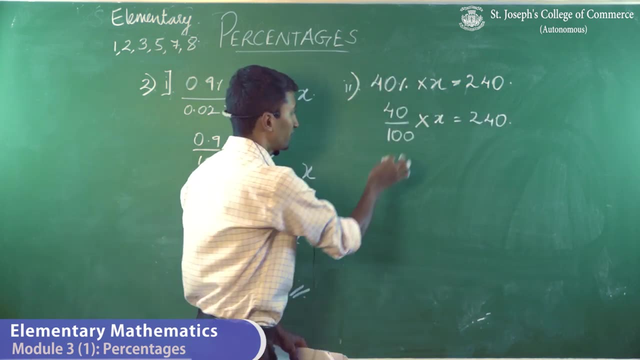 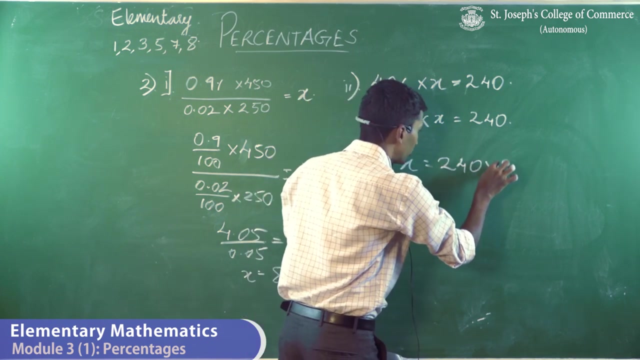 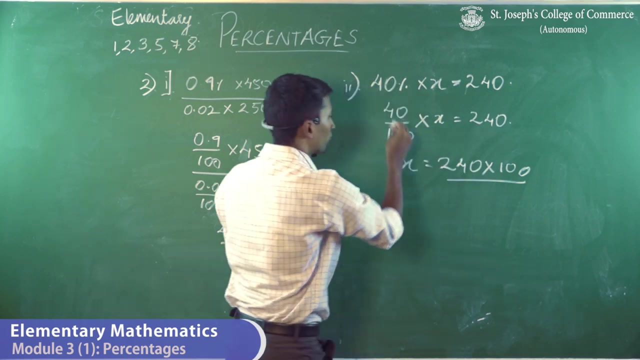 So what we do is 40%. so 40 by 100 of X is equal to 240. So we take 40 by 100 to the other side. So all we have to do is 240 into 100 goes up as a numerator and 40 comes down. 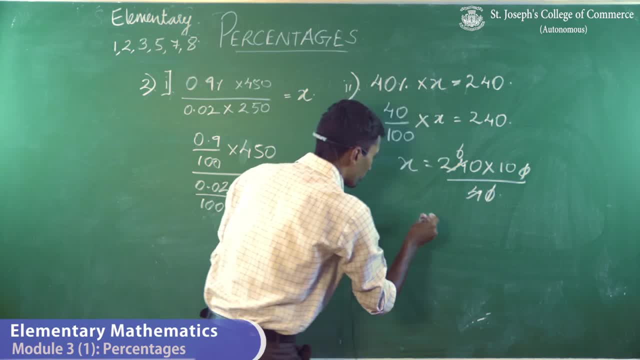 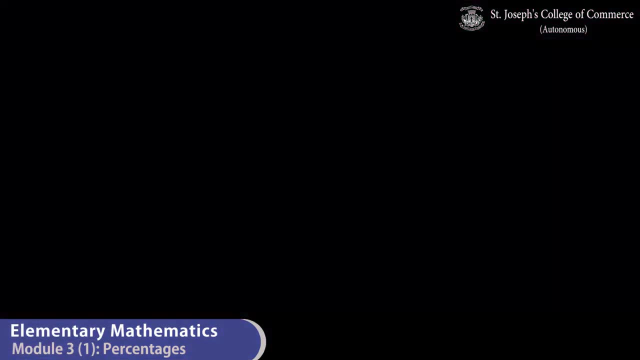 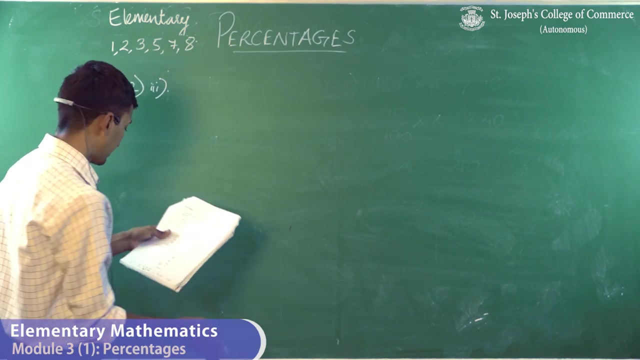 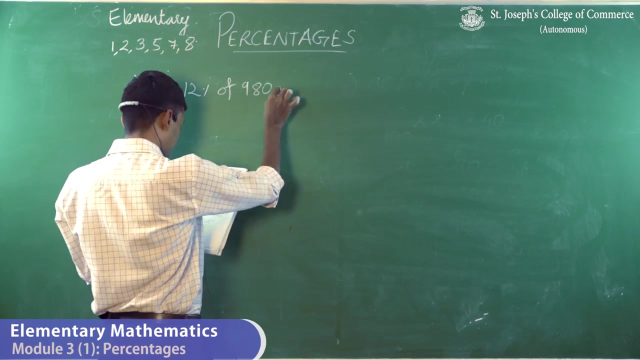 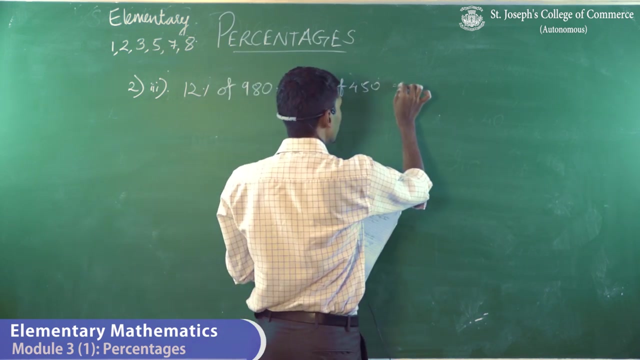 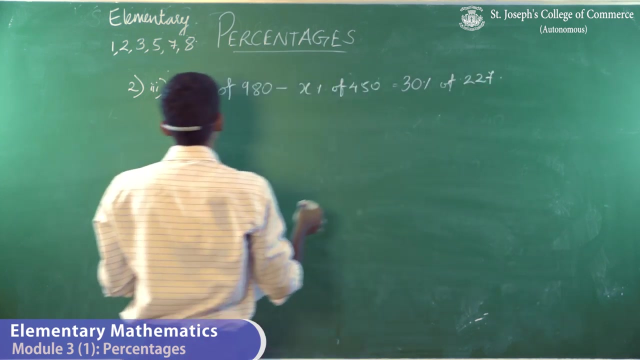 as the denominator. If you solve it you get: X is equal to 600.. We now move on to the second sum, third part, where in the result they say: 12% of 980 minus X% of 450 is equal to 30% of 227.. 12% by 120 of 980. 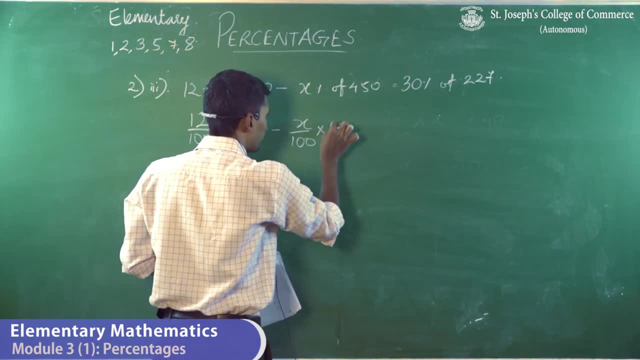 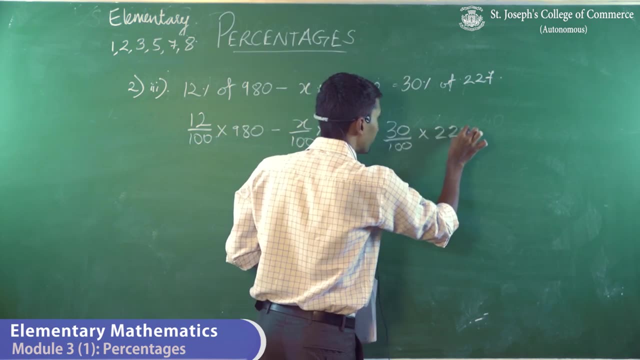 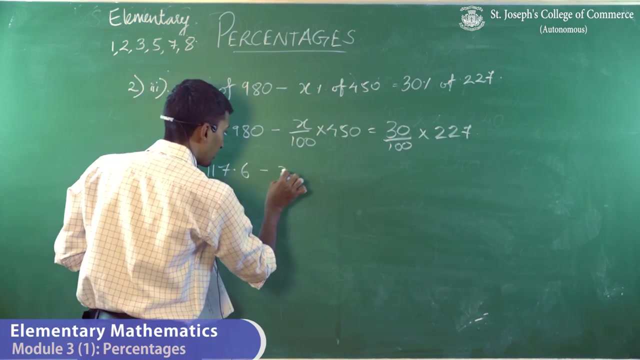 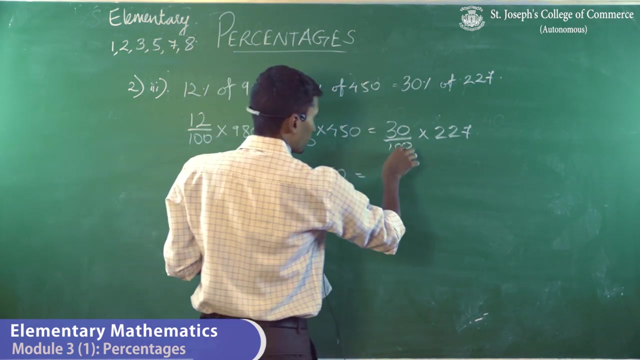 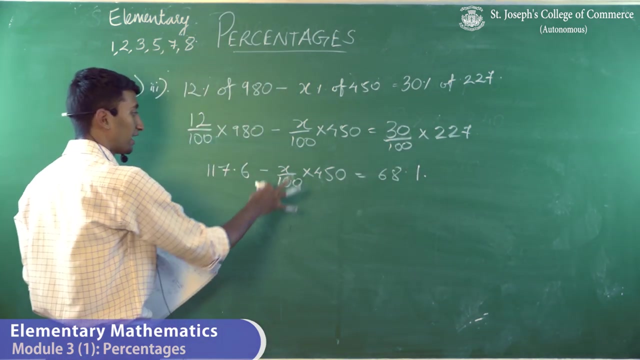 minus X by 100 is what we got. 12% by 120 is equal to 207.. of 450 is equal to 30. by 100 into 227, this will give me 117.6. minus x by 100 into 450 is equal to 68.1. so now bringing 68.1 this side and putting the x on the other side, 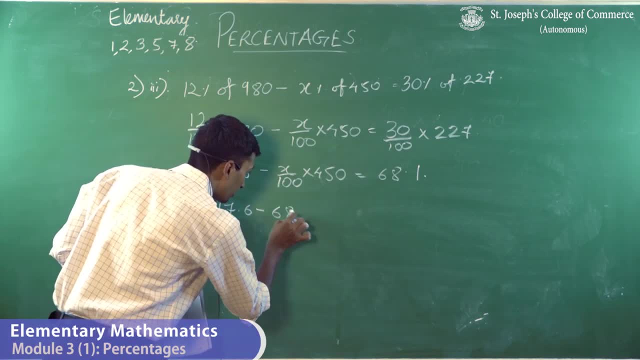 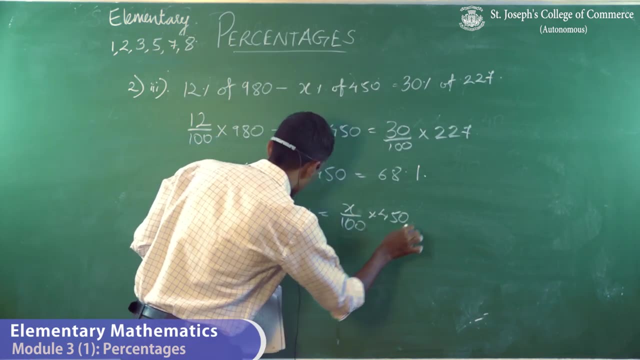 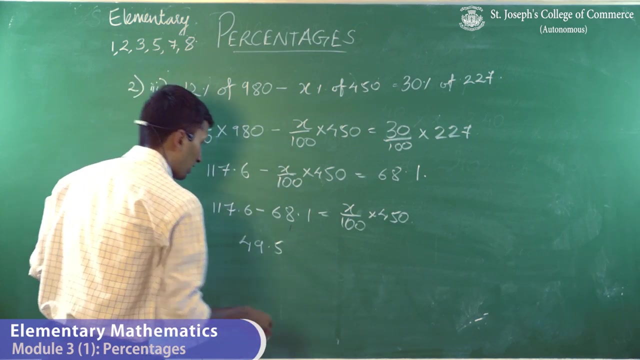 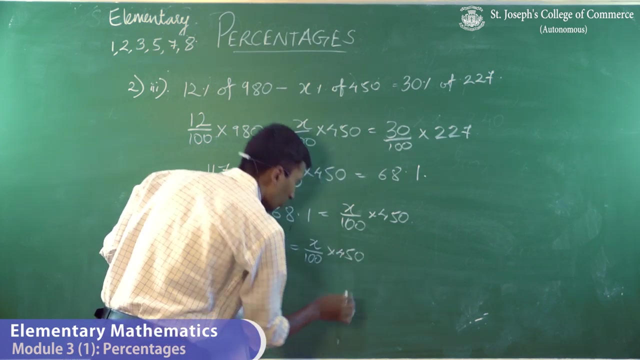 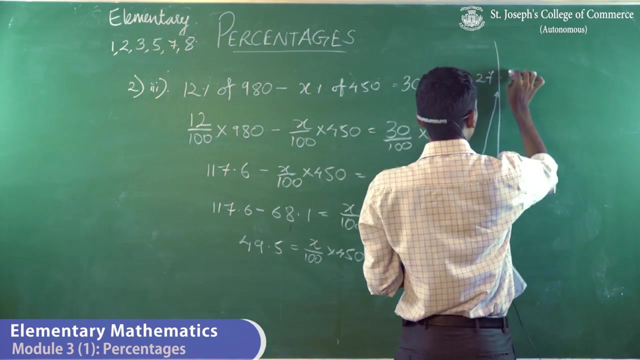 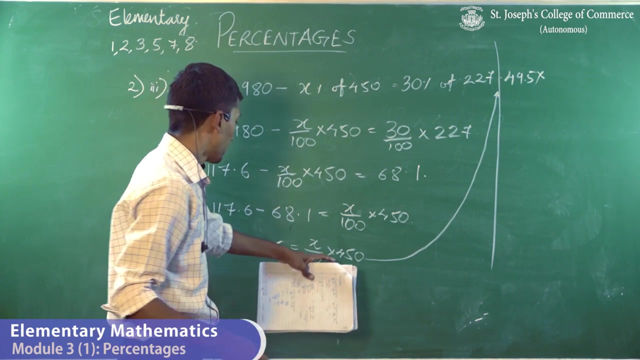 bringing the constants onto one side, plus x by 100 into 450, so that would be 49.5- is equal to x by 100 into 450. taking it to the other side, 49.5- we're taking 450 and 100 onto the other side, so that would be a 100, which is in the denominator. 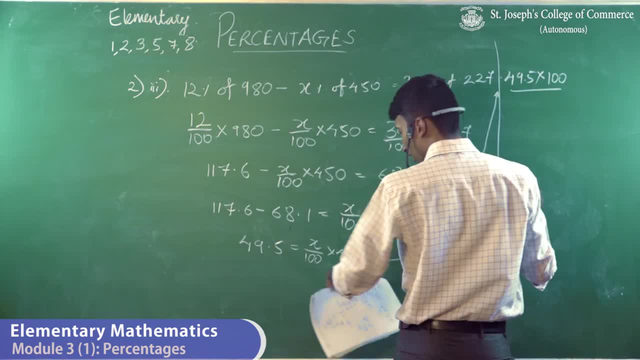 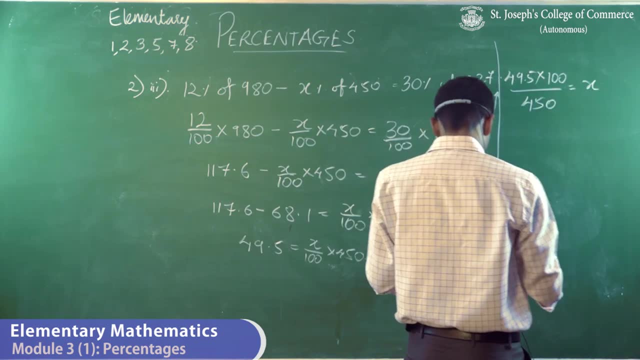 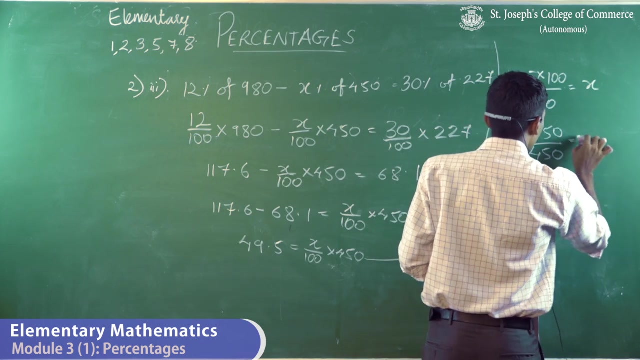 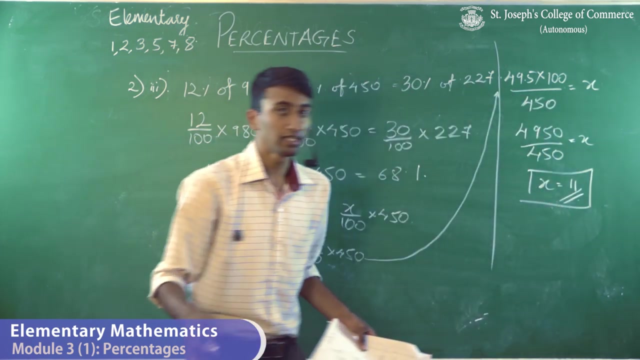 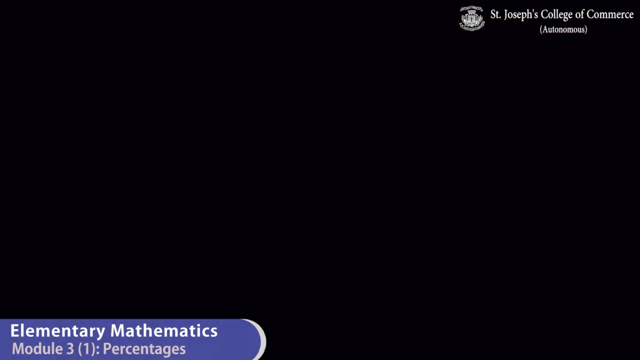 will go into the numerator into 100 divided by 450.. 450 comes in. the denominator is equal to x, so that would be 4950 by 450 is equal to x, and so x is equal to 11, so x is 11. so now some number. 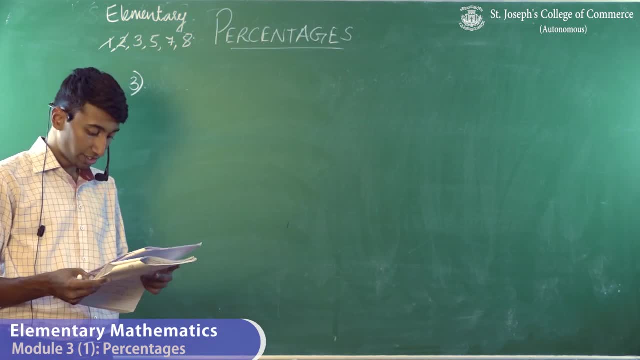 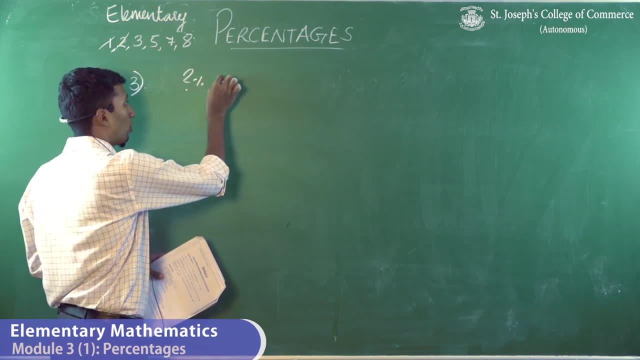 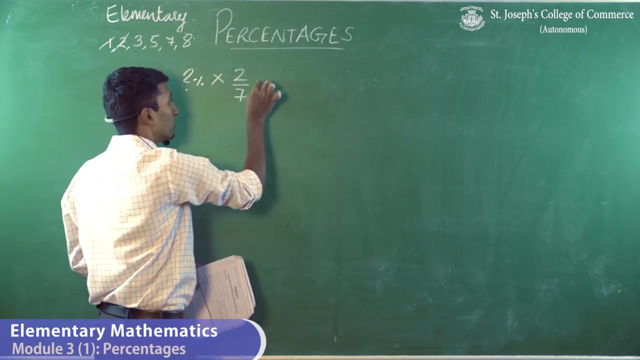 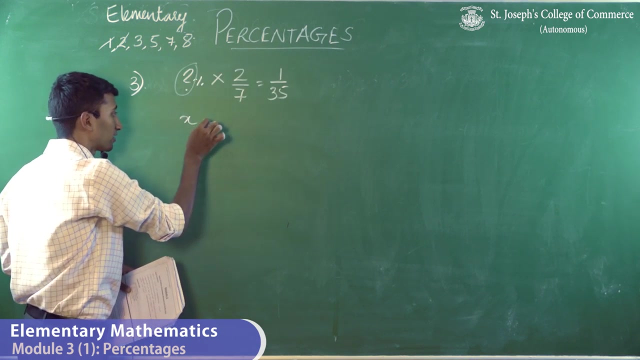 3, some number 3 says what percentage of 2 by 7 is 1 by 35. so what percentage of so off is always a multiplication of 2 by 7 is 1 by 35. so this question mark I will replace it as x, so x percentage of 2 by 7.. 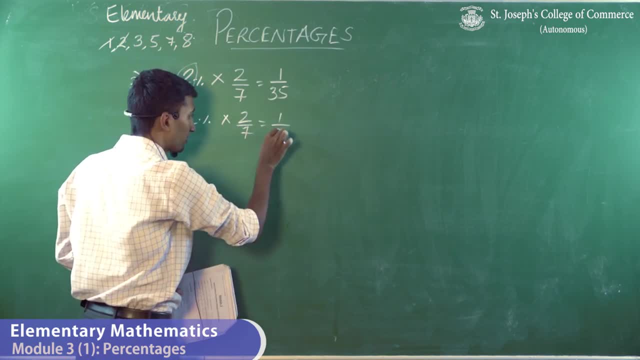 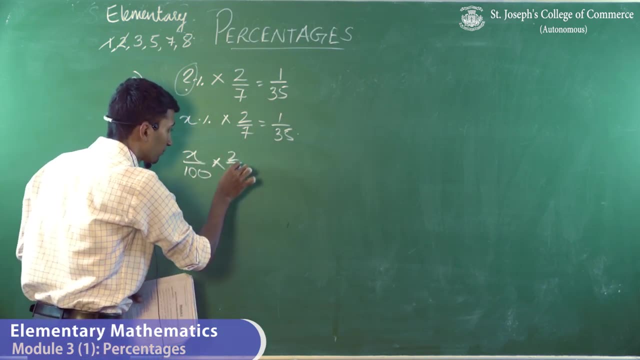 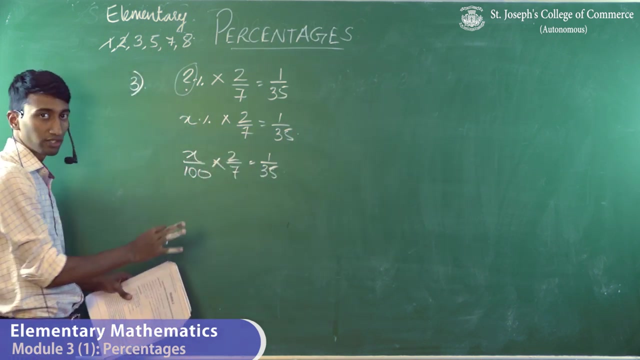 2 by 7. is equal to 1 by 35. so x by 100.. is into 2 by 7. is equal to 1 by 35. which I would take all the constants onto one side and keep x on the site, so that would. 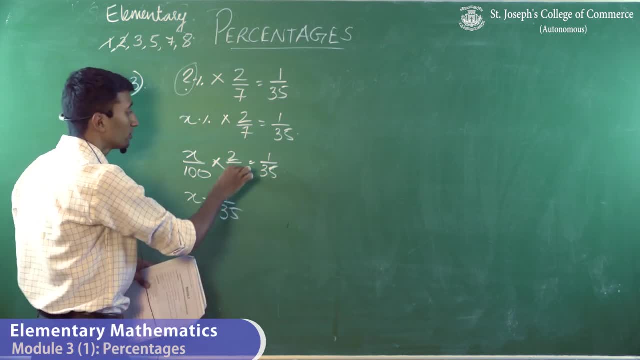 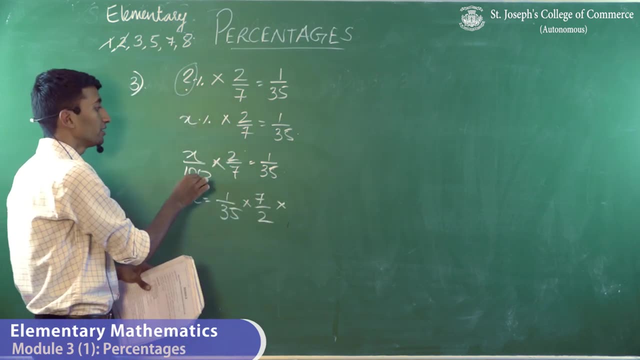 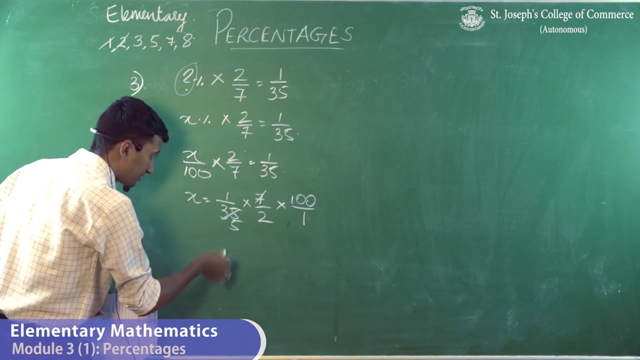 be 1 by 35.. 7 goes into the numerator and 2 comes into the denominator, so 7 by 2.. into, since hundred is in the denominator, goes into the numerator hundred by 1.. so 7, 5 or 35.. 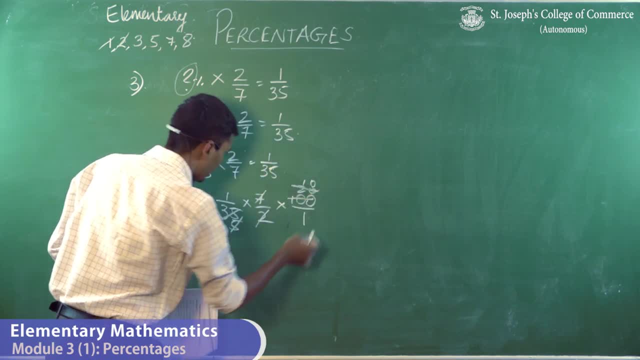 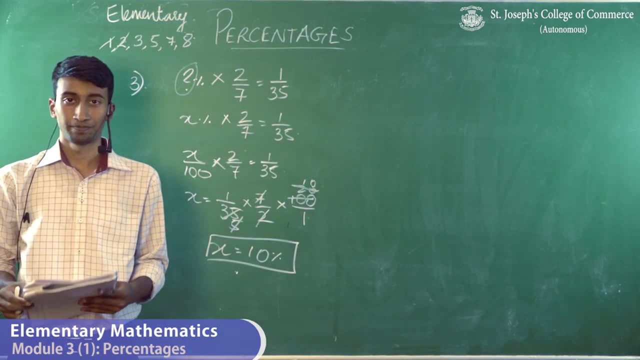 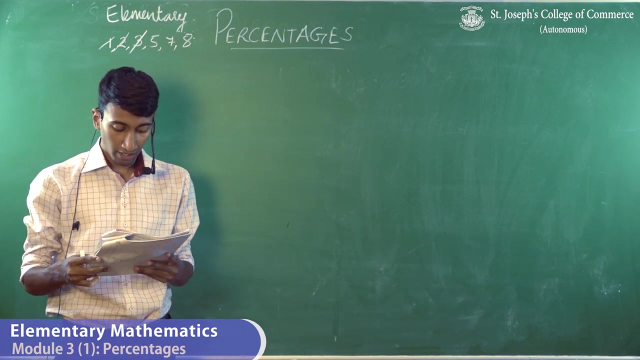 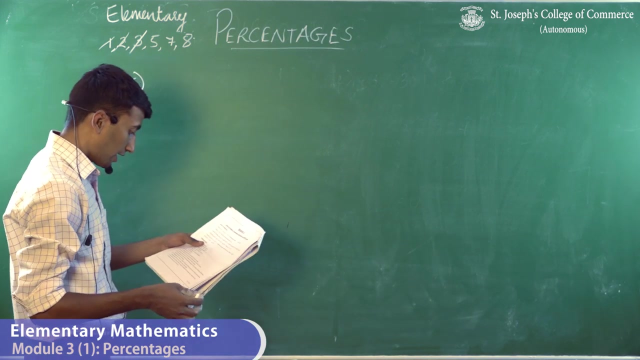 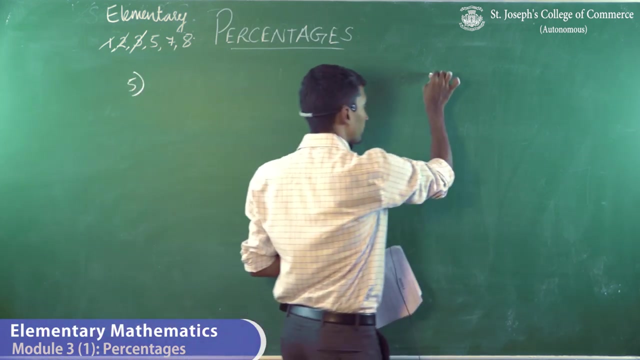 5- 2s are 10, so 20.. 2- 10s are 20, so x is equal to 10%. the fifth sum states that sixty five percent of a number is twenty one less than four fifth of that number. find the number. So I'll give you an example: 10 is less than 12 by 2.. So 10 is less than. 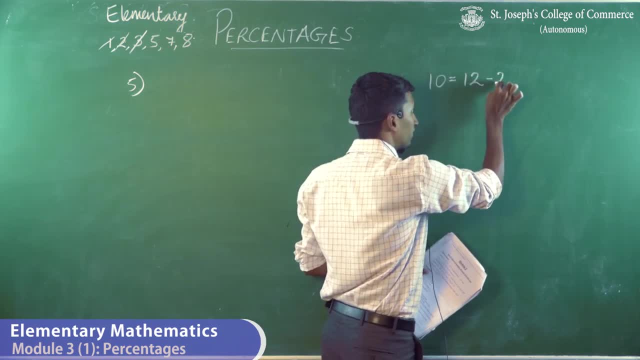 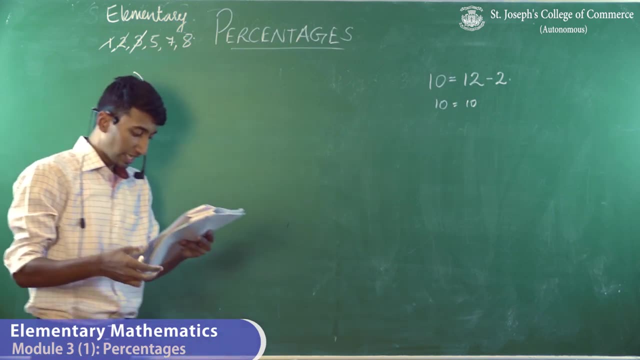 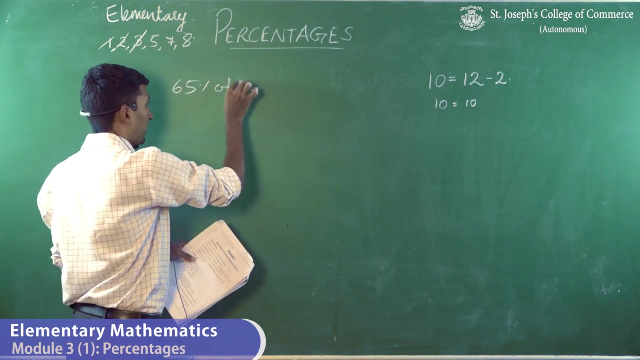 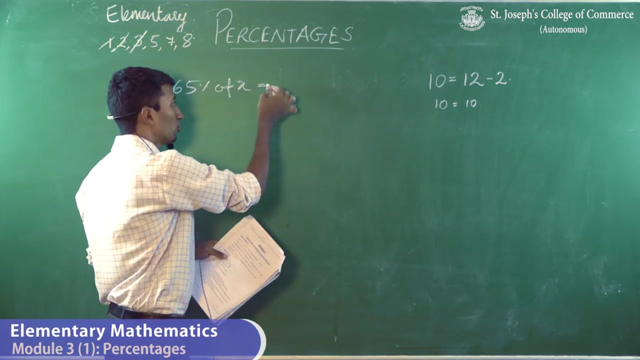 12 by 2. So that means 10 is equal to 10.. Same way, 65% of a number, so 65% of x, is 21. less than 4 fifths of that number, So it is less than. 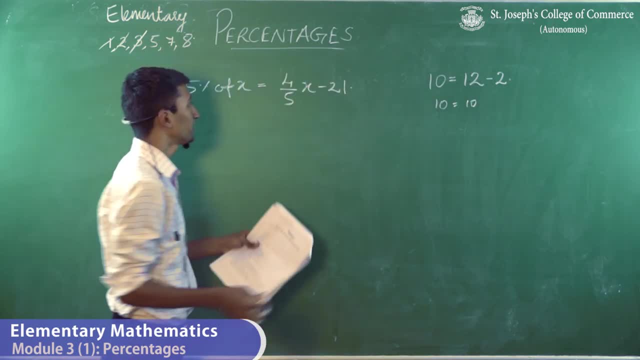 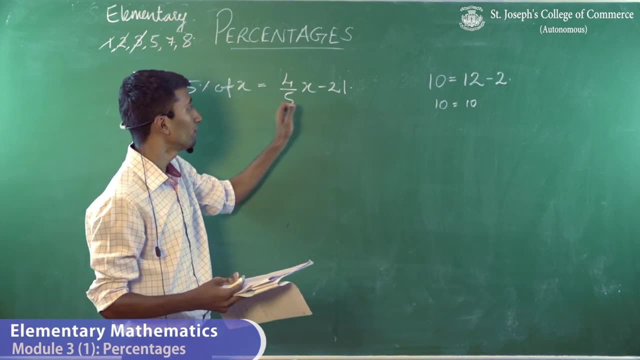 1. So basically, what they're trying to say over here is it is 21 less than 4 fifths of that number. So that means this 4 fifths of the number is 21 more than this side. So to make: 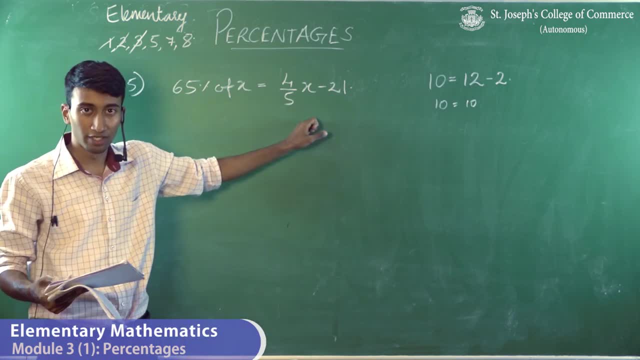 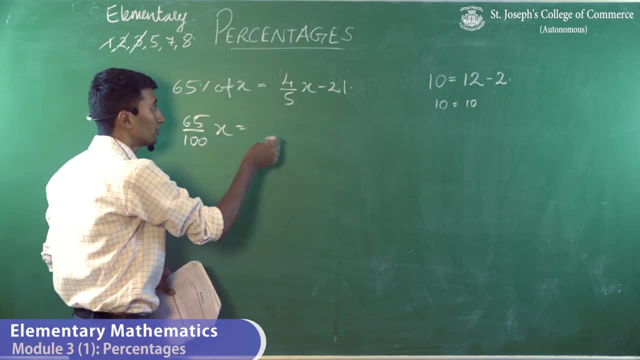 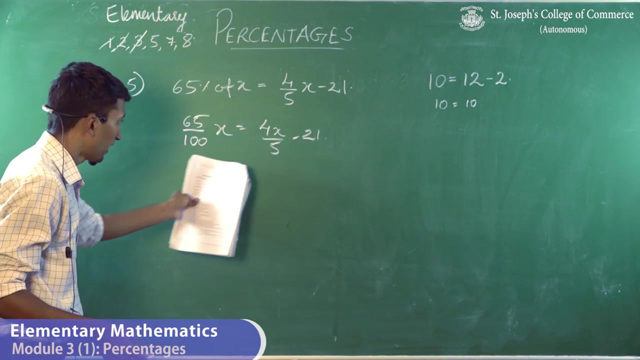 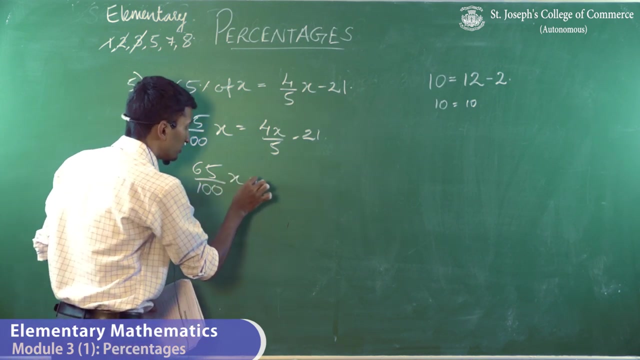 it equal. I minus 21 from this side, so that it's equal. So now, if I solve it, it becomes 65 by 100 x is equal to 4, x by 5 minus 21.. Okay, Now, getting the x onto one side, it is 65 by 100. x is equal minus 4 by 5, x is equal. 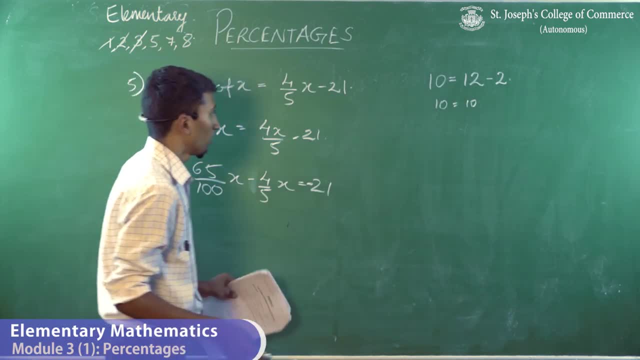 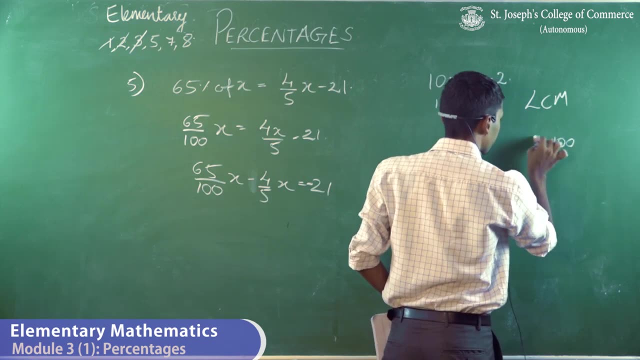 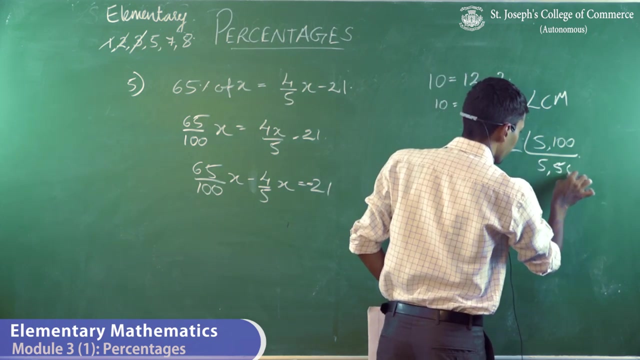 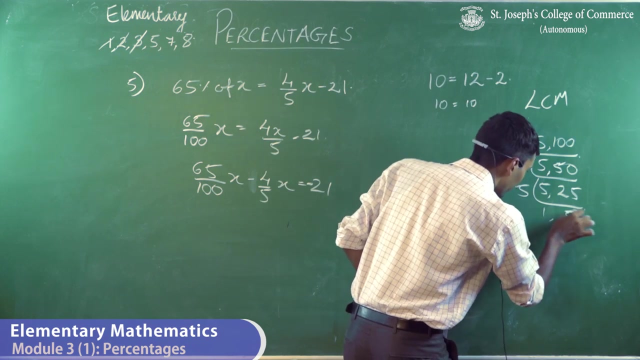 to minus 21.. So now, taking the LCM, it is 105.. So 5,, so 2.. 50. And divided by 2 again 25.. 5 ones are 5, fives are and 5 ones are Okay. So now. 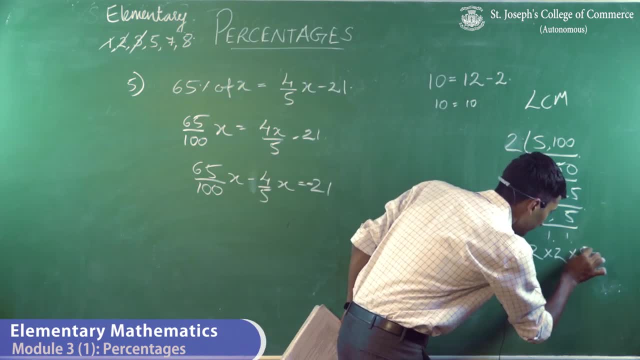 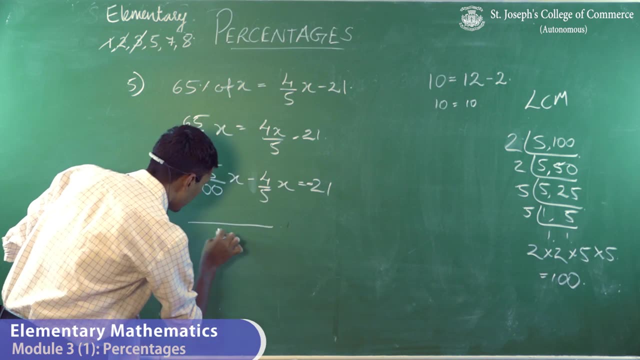 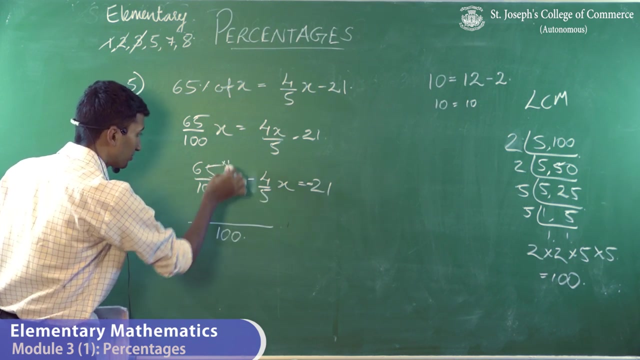 2 x 2 x 5 x 5 will give me 100.. So LCM over here is 100.. So, taking LCM as 100, this is multiplied by 1.. So 65 is multiplied by 1. So that's 100.. So that's 100.. So, taking LCM as 100, this is: 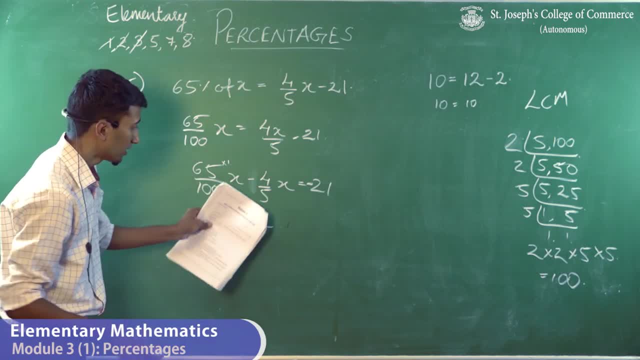 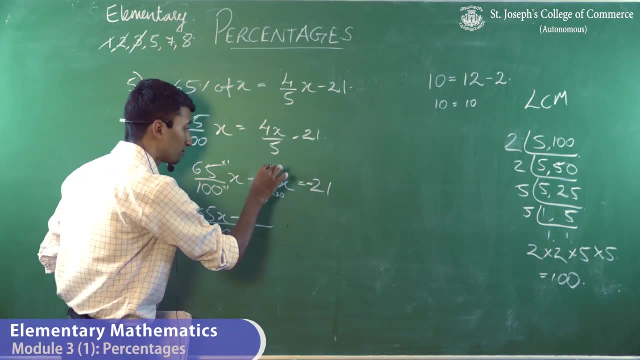 multiplied by 1.. So 65 x minus 5 watts are 100.. 5 x 20 will give you 100.. So if you're multiplying the denominator by 20, you have to multiply the numerator also by 20.. So that: 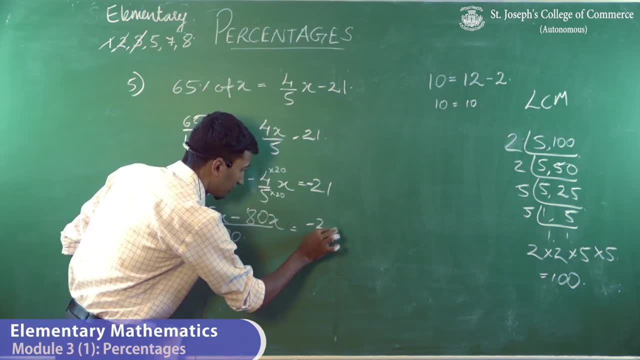 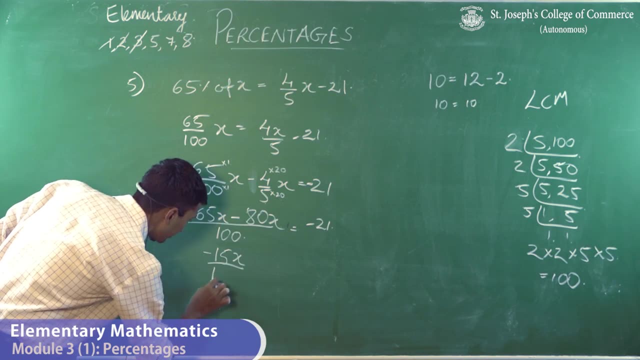 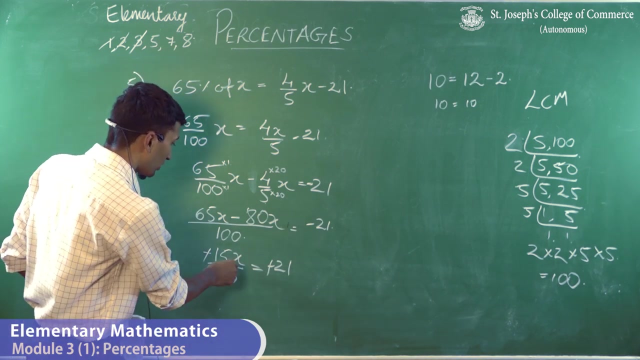 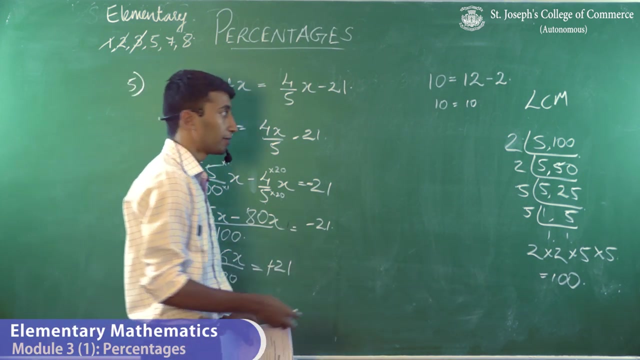 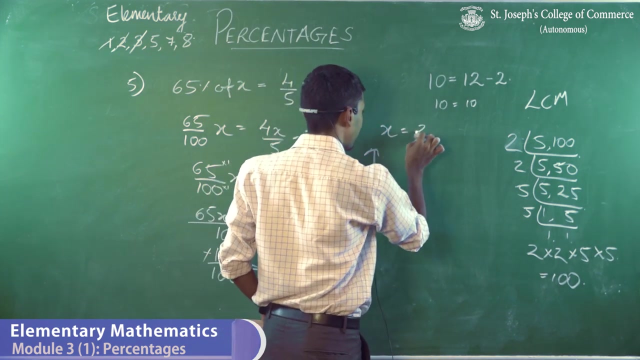 would be 80. x is equal to minus 21.. That would be minus 15. x by 100 is equal to minus 21.. Cancel out the minus signs And so keeping the x on this side, on the left-hand side, and transferring the values onto the right-hand side, it becomes x is equal to 21 into. since 100 is in the denominator, it goes into the numerator. 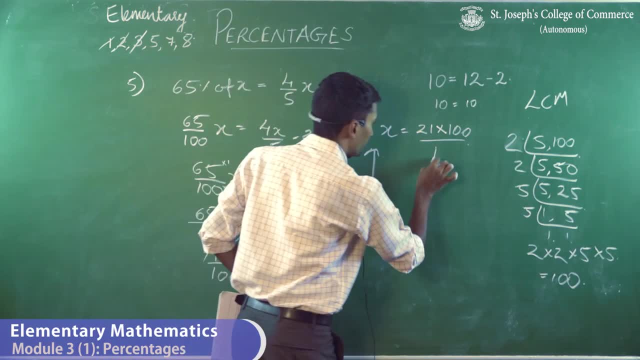 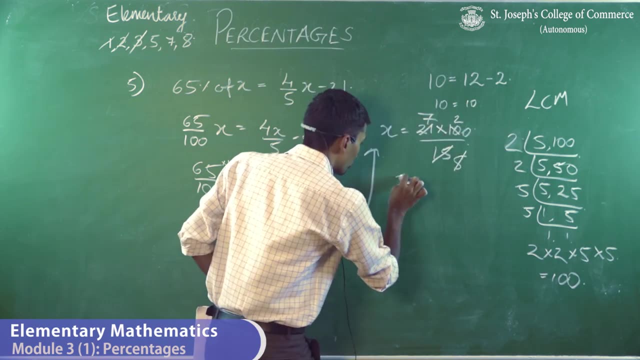 And since 15 is in the numerator, it comes into the denominator. So three 5s are 15, three 7s are 21.. Five 2s are 10.. So x is equal to 140.. So that is your answer. 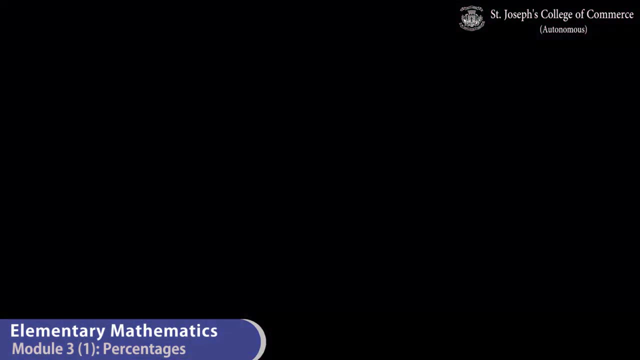 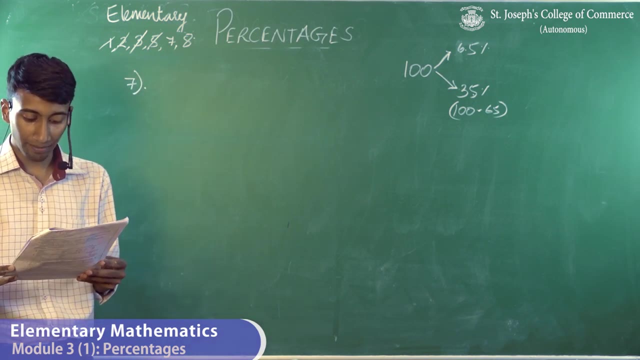 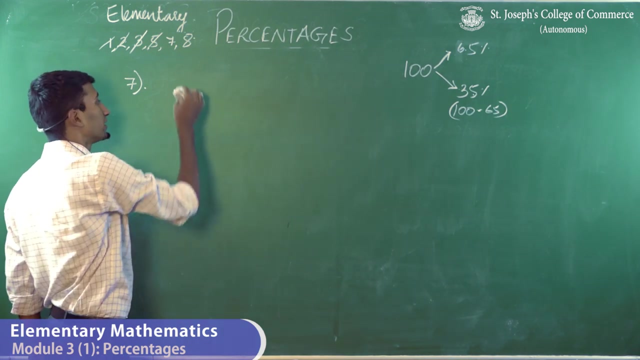 That's the variable you need to find. Moving on to the seventh sum, it states that in an examination, 65% of the total examinees passed. If the number of failures is 420, find the total number of examinees So over here. since they're asking you to find the total number of examinees, that is the variable. 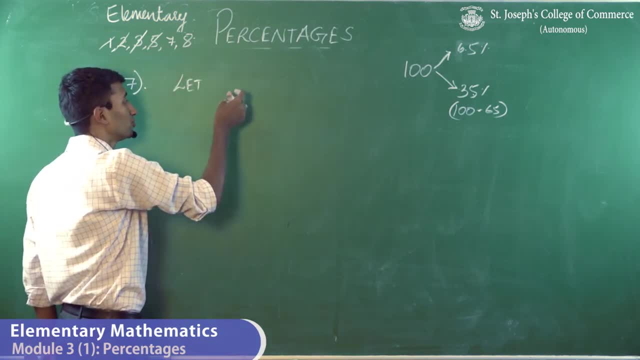 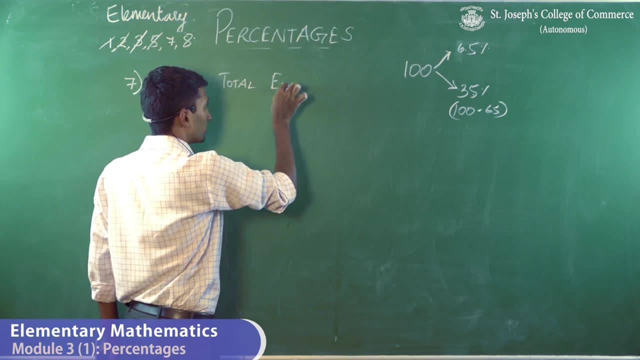 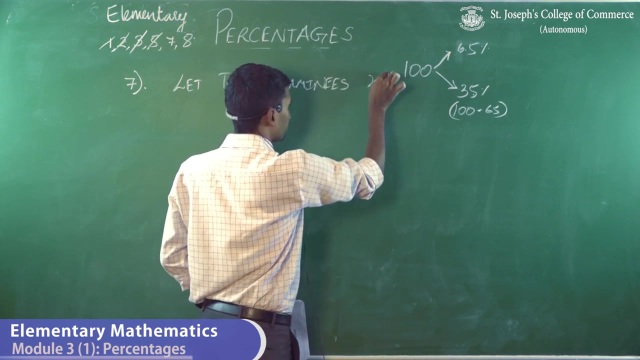 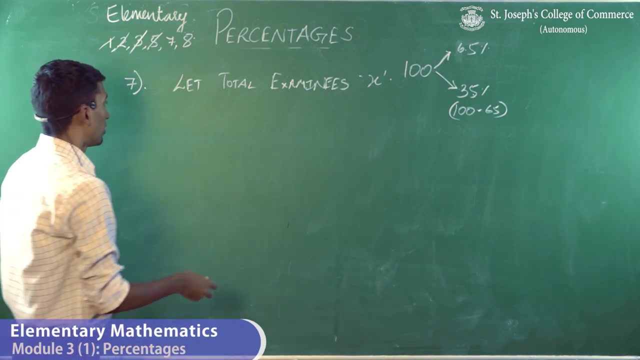 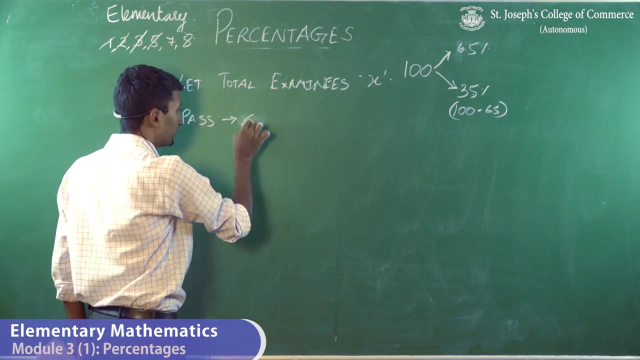 That you do not know. So you assume, let total number of examinees be x. Yeah, So since the total number of examinees is x and you know that pass percentage is 100, is 65%. So out of 100,, 65% of them passed. 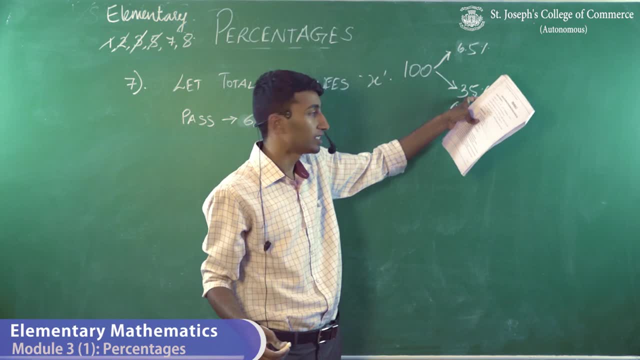 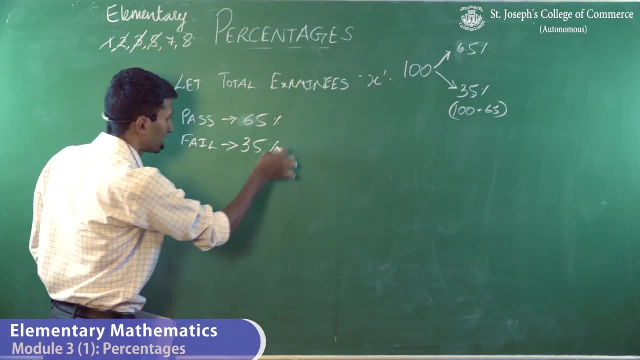 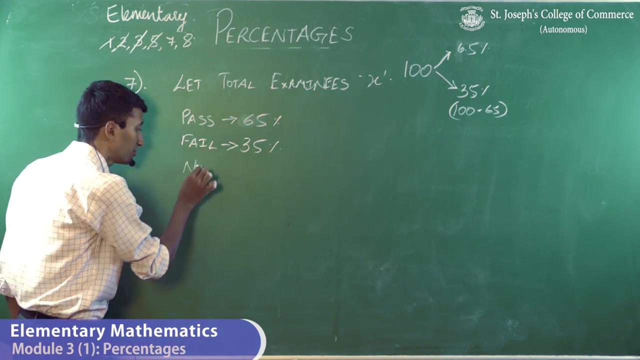 So the remaining 35%, 100 minus 65 is 35%. So the remaining failed, So the failed percentage is 35%. So now, if you know that the percentage, the failed percentage, is 35, and you also know the number of people who failed, 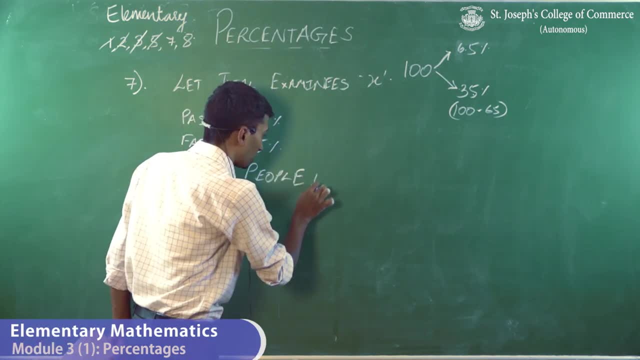 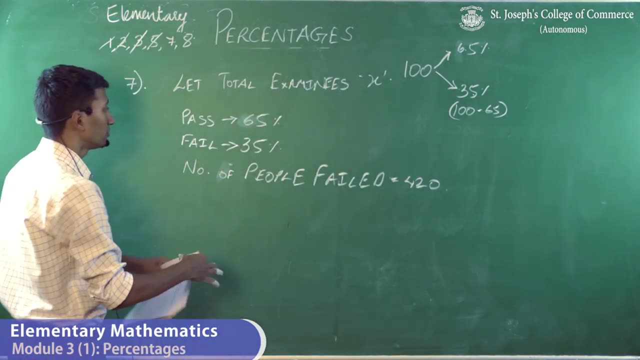 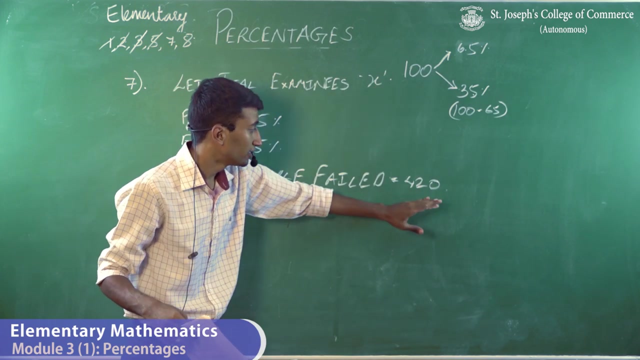 People failed is 420.. So all you need to do now is since. so all you need to do is 35% of the total number of examinees failed. So 35% of x is equal to 42, because this is the number of people who failed as well. 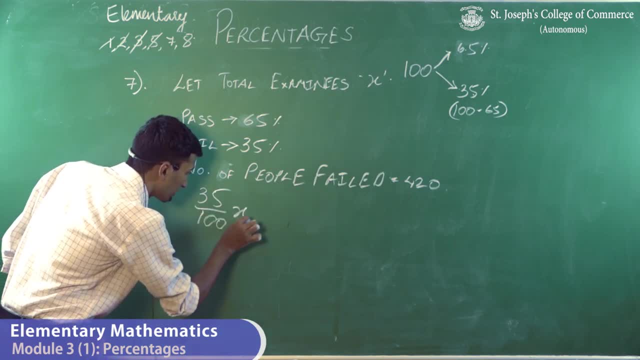 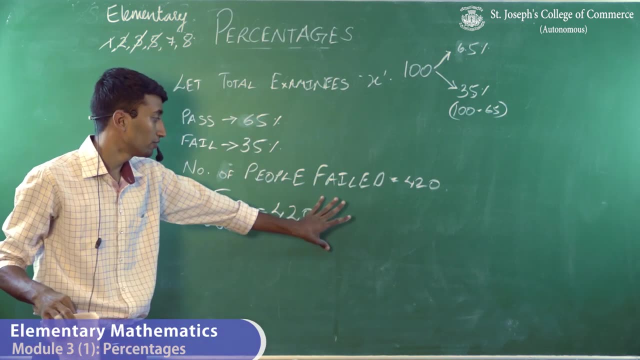 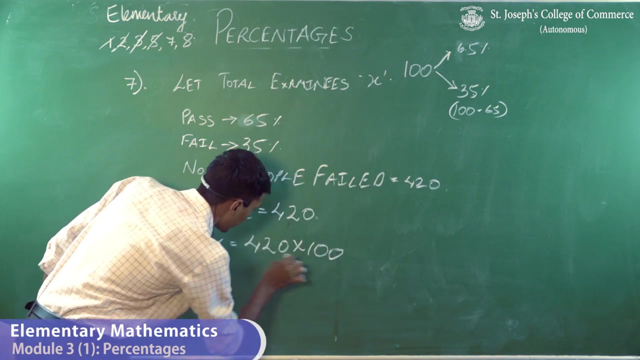 So 35% of x is 420. So keeping the number, keeping x. So just by going on the left-hand side and transferring the values on the other side, x is equal to 420 into 100 divided by 35.. 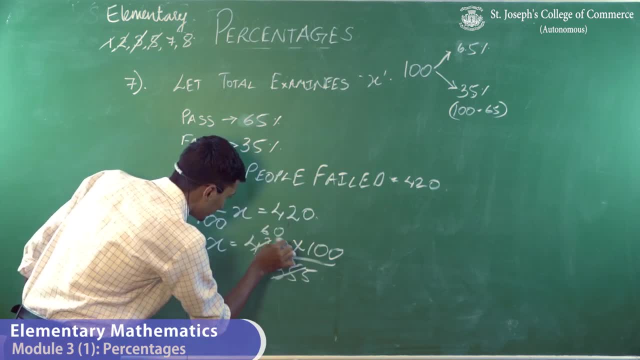 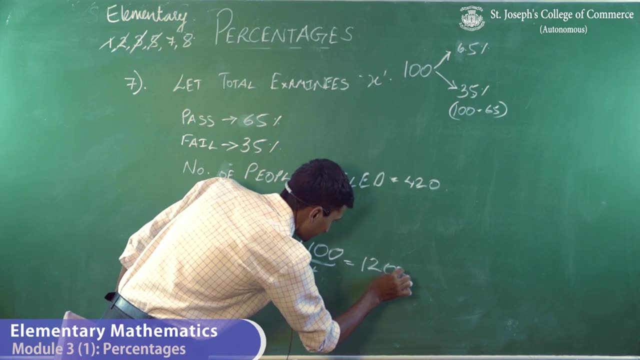 Five are 35,, six are 42,, so 60. Five 12's are 60. And so 12 into 100 will give me 1,200.. So the total number of examinees the answer at the end of it. of examinees is 1200..